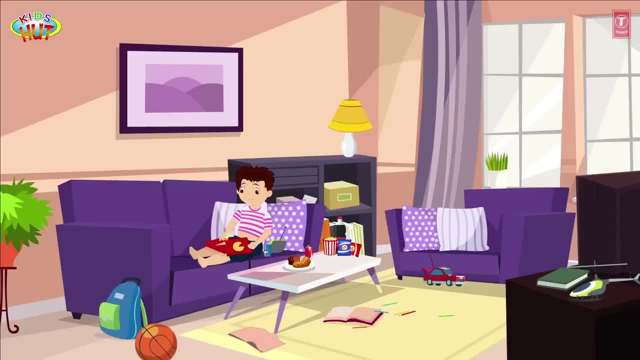 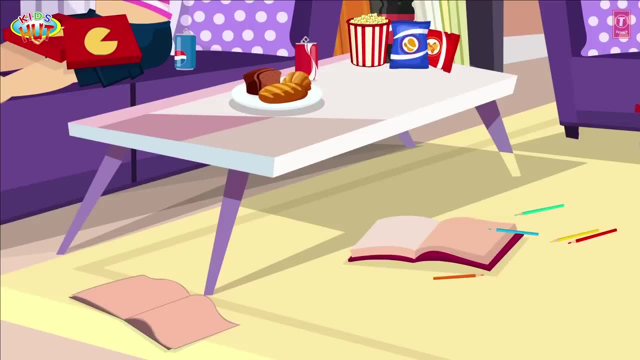 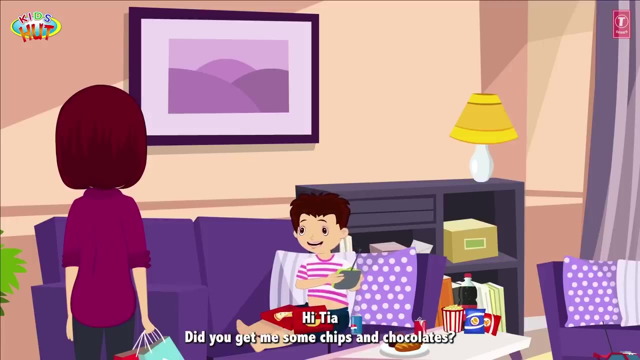 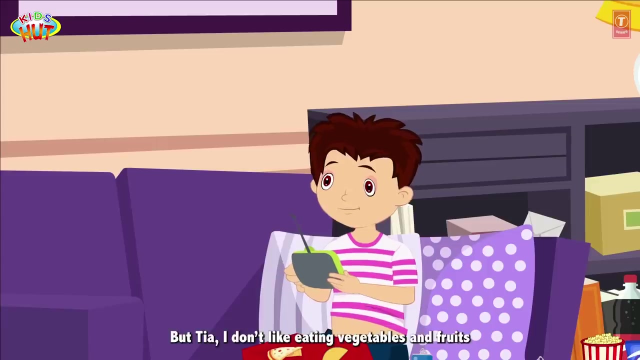 Join Kids Heart Family. Oh dear, What a mess you have made. Hi, Tia, Did you get me some chips and chocolates? No Tofu. You're eating a lot of junk food these days, But, Tia, I don't like eating vegetables and fruits. 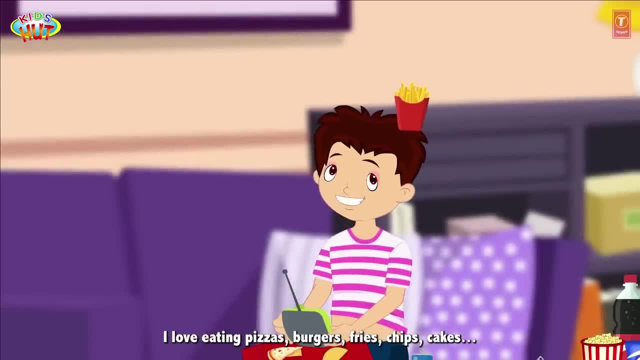 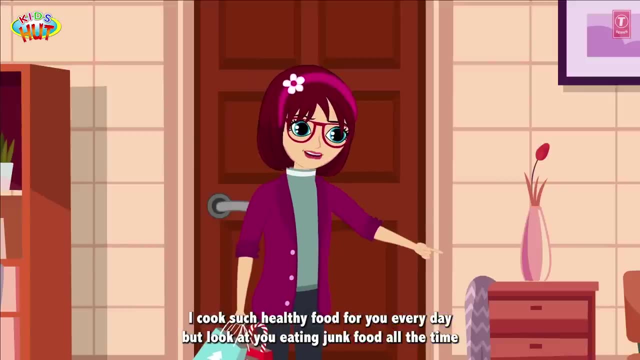 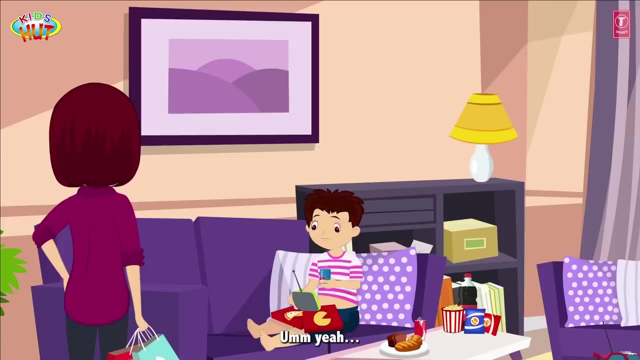 I love eating pizzas, burgers, fries, chips, cakes. I cook such healthy food for you every day, But look at you eating junk food all the time. It's so harmful for the body and your health. Hmm, Yeah, Tofu. clean this mess and complete your homework. 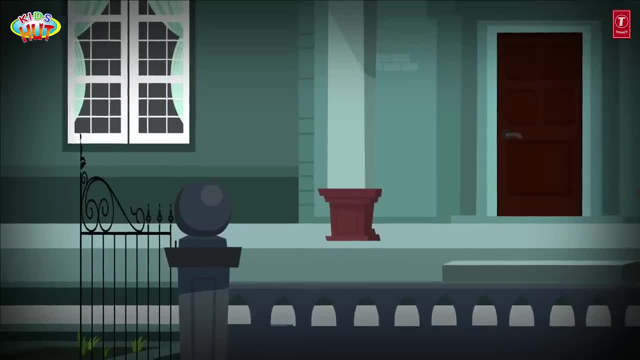 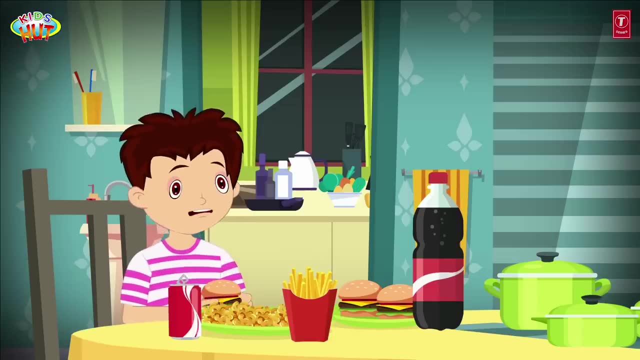 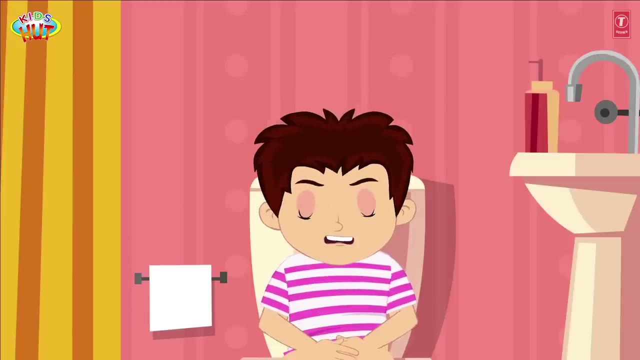 I will. I will, Tia, Don't worry. You don't have to worry, I'll take you to the hospital. Tofu is everything alright? No, Tia, My stomach hurts so much I feel sick. 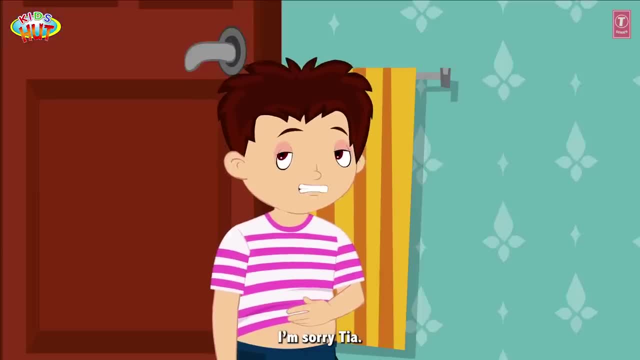 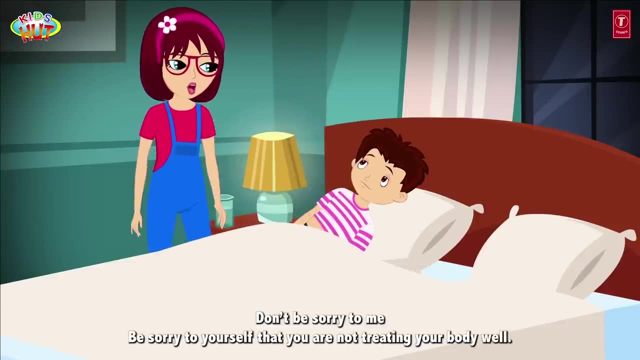 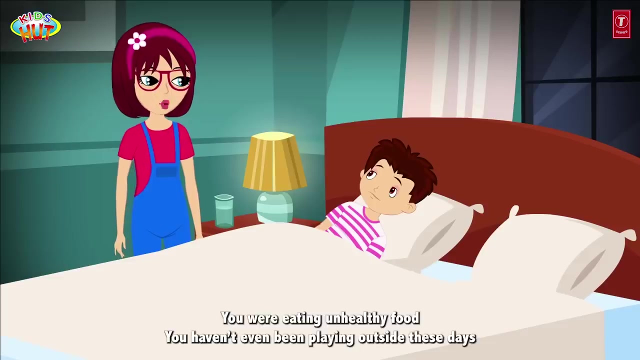 Oh, Tofu. I told you not to eat all that junk food that you've been eating since so many days. do now, don't be sorry to me. be sorry to yourself that you're not treating your body well, Tia, but how did? I felt sick because of food you were eating- unhealthy. 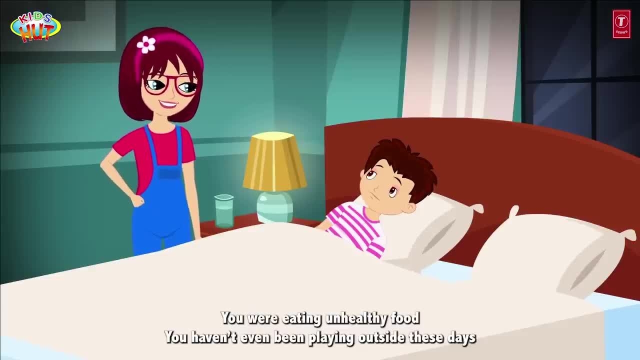 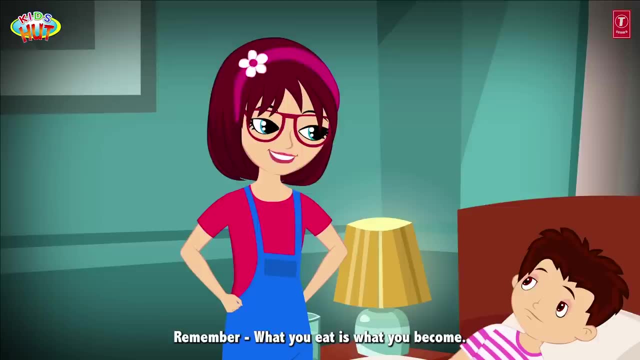 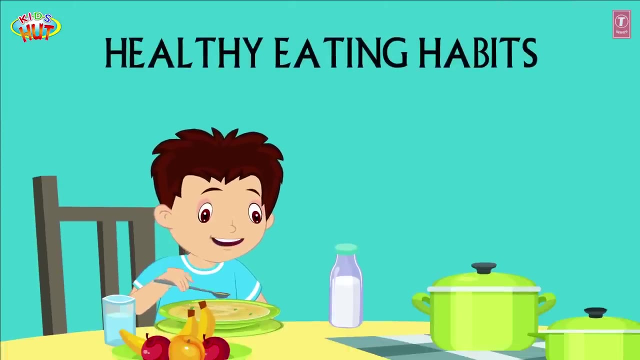 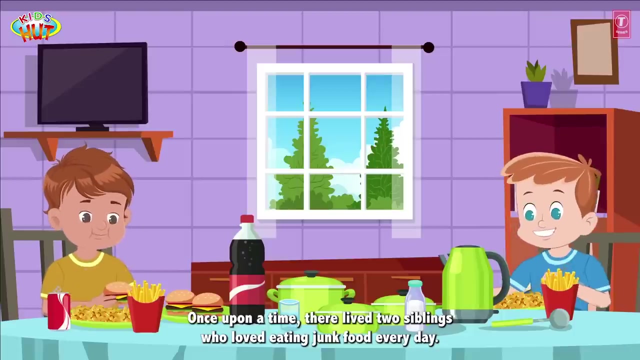 food. you haven't even been playing outside. these days, good food and exercise are so important for your body. remember: what you eat is what you become. what does that mean, Tia? healthy eating habits. once upon a time there lived two siblings who loved eating junk food. every day, they refused the healthy meals. 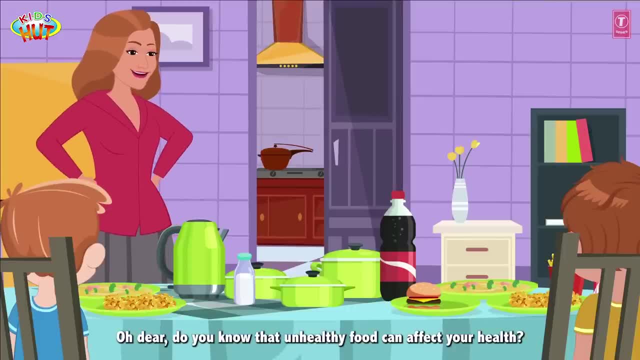 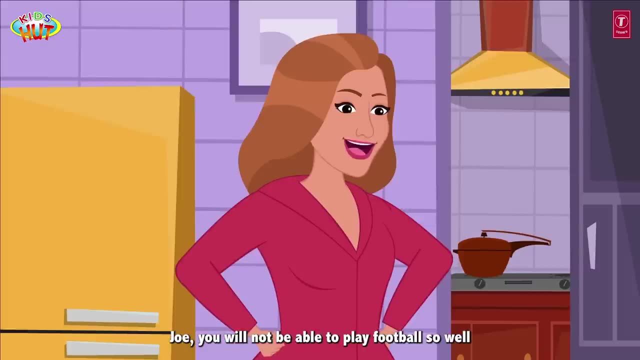 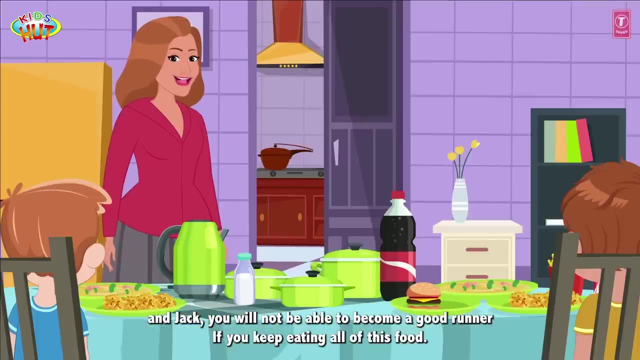 that their mother cooked for them. oh dear, do you know that unhealthy food can affect your health? Joe, you will not be able to play football so well and Jack, you will not be able to become a good runner if you keep eating all of this junk food. but, mom, this tastes so good. I cannot eat these fruits and